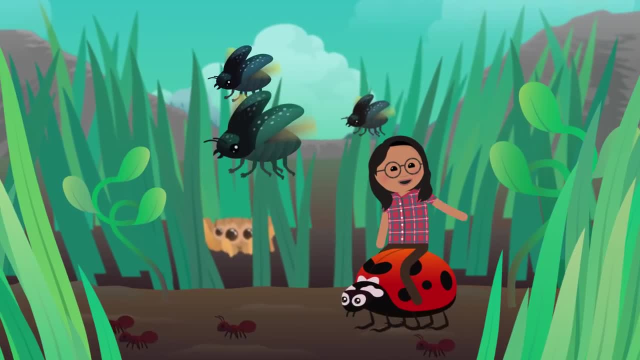 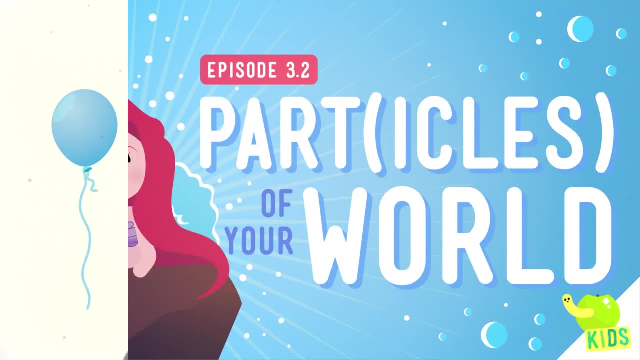 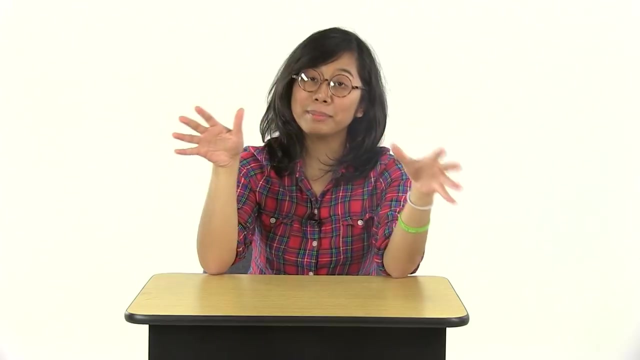 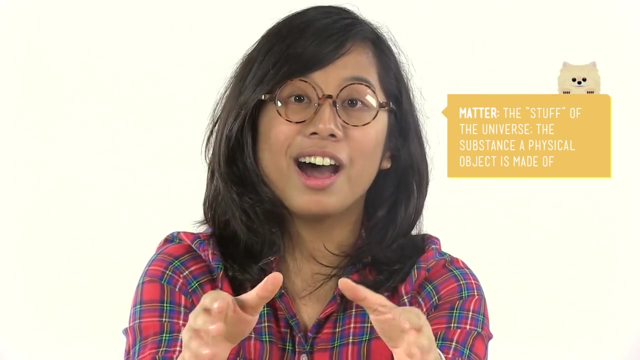 You ever hear someone say: you look like a million bucks. Well, you do, But you also look like a million particles. Let me explain. You and I are both made of matter. I don't mean we matter like we're important, even though of course we are. I mean we actually. 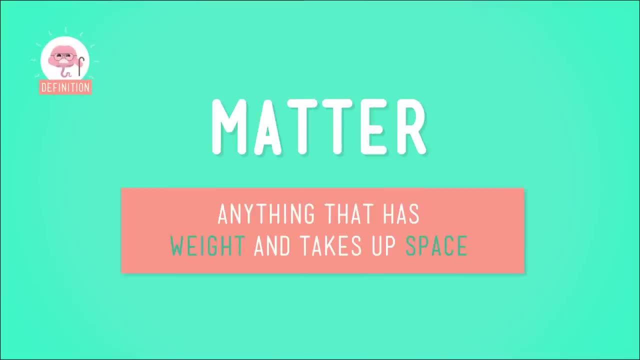 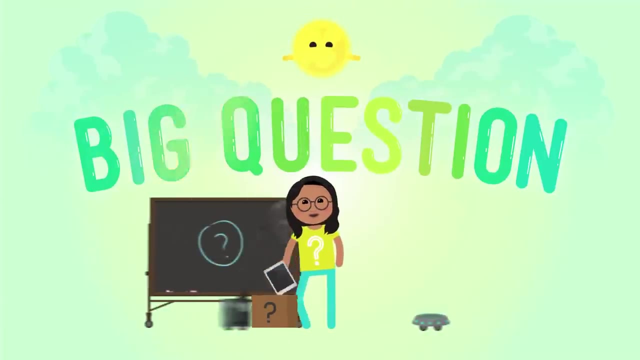 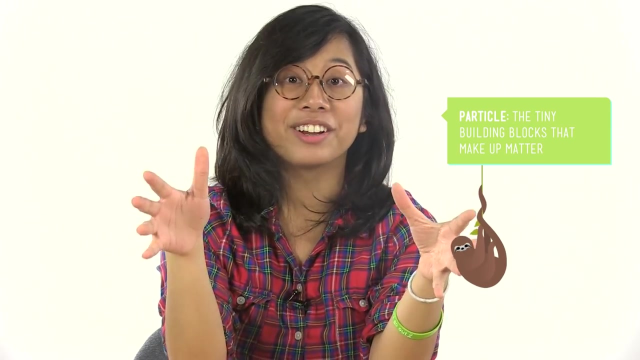 are matter. Matter, as you know, is anything that has weight and takes up space, And we did a whole video about it. But what is matter made of? It's made of particles. So you, as a big thing of matter, are made of particles. The device you're watching this on is made. 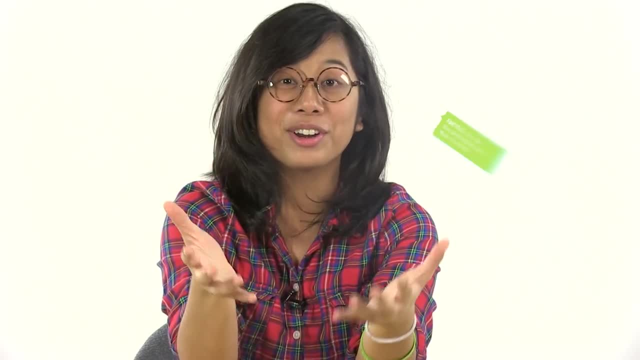 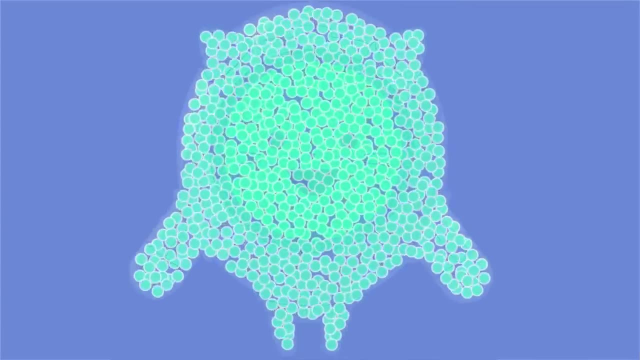 of particles. Your dog is made of particles. You get the idea. Particles are so tiny though You can't see them. Just picture them as super small balls packed together to form an object. And how an object looks and behaves, which we call its properties, has a lot to. 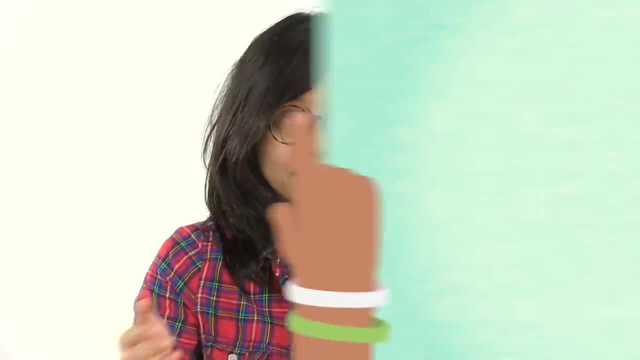 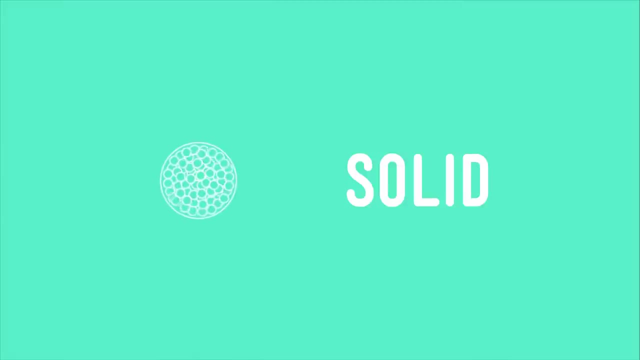 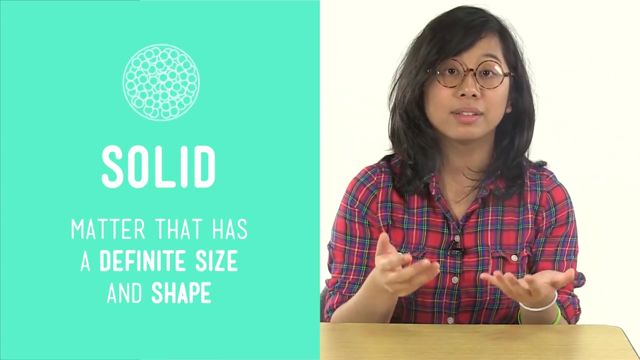 do with those tiny particles that it's made of. Let's take a look. You know that most matter comes in three states: Solid, liquid or gas. Particles in a solid are packed so tight that they don't move And they keep you from moving through it Like a brick wall. 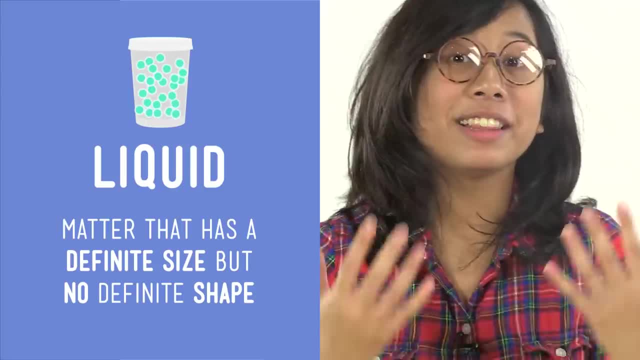 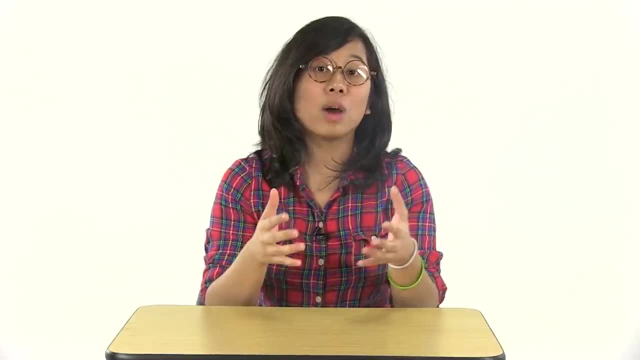 Now, don't try running through a brick wall, Just trust me on this. But in a liquid there's more space between the particles. That extra room between them allows them to slide around. That's why you can stick an object into or through a liquid, like dropping a straw in a glass of soda or wading through a pool. 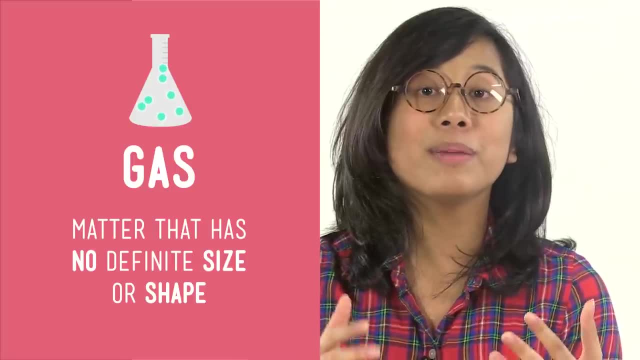 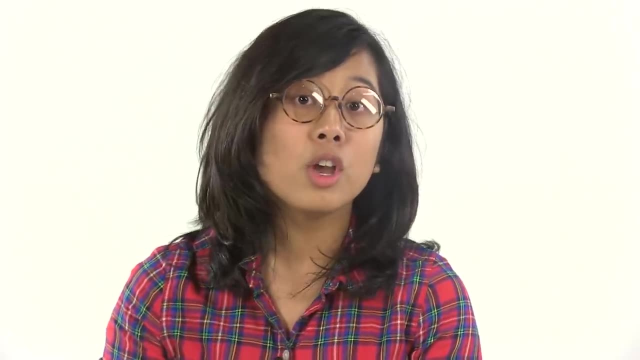 of water And there is so much space between the constantly moving particles in a gas that you can move around in them easily. In fact, when you walk from one side of the room to the other, you've walked through a bunch of gases that make up air. But if something, 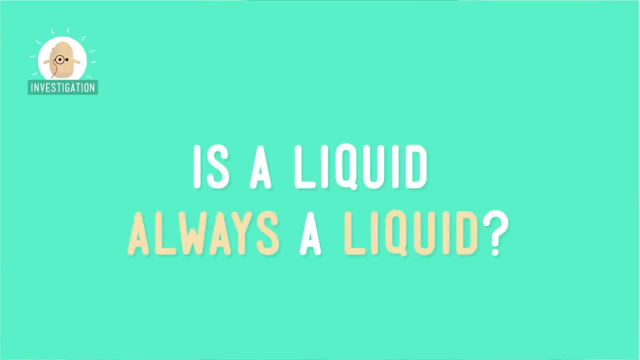 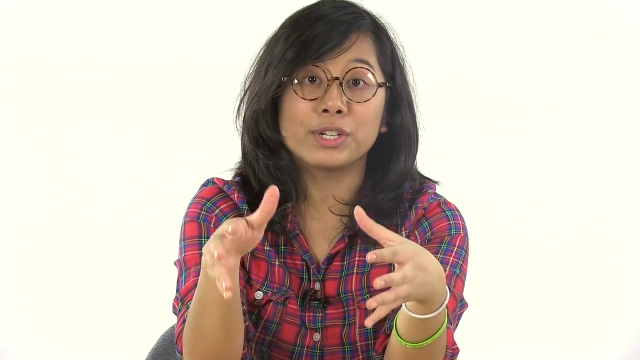 is a solid, will it always stay a solid? Well, that's a good question. But if you're a solid, is a liquid always a liquid? Do gases ever become non-gases? To find out if matter can change states, let's find examples of when objects' properties.